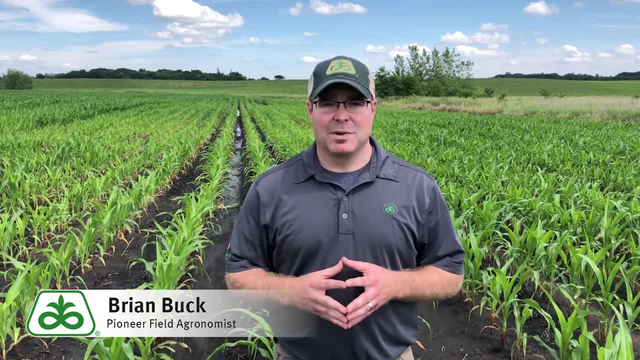 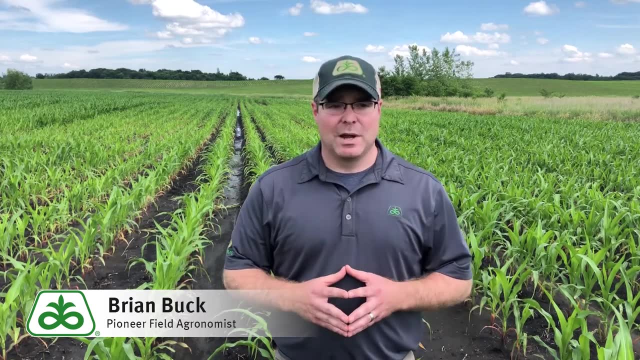 it does pay to go and rescue apply on those areas that have lost quite a bit of nitrogen. If you look out into this field here, you can kind of see that yellow hue coming up and this is probably an extra wet situation, but this would benefit from a little bit of nitrogen.